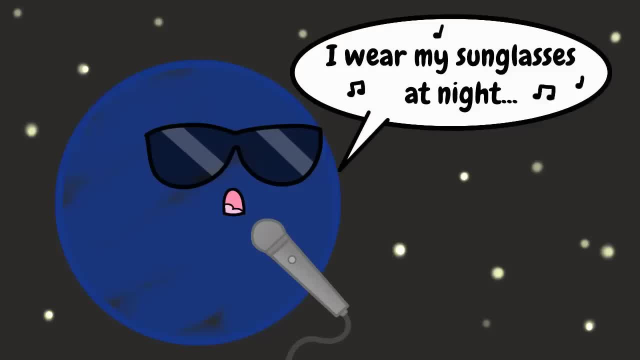 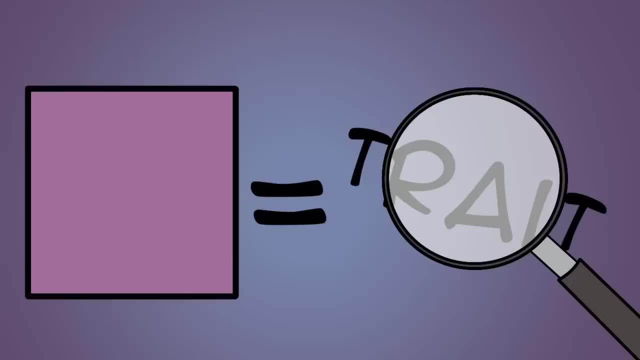 there are two children from this marriage. Now you may wonder: why are some of these shapes shaded? What does that mean? Well, the shaded shapes represent a trait that is being tracked in the pedigree. Here are two important facts about the particular trait I am choosing to track: Fact number. 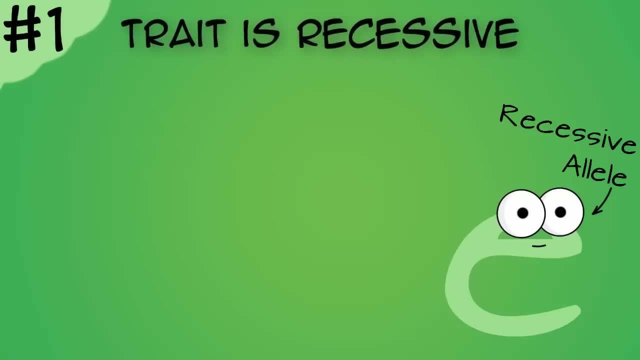 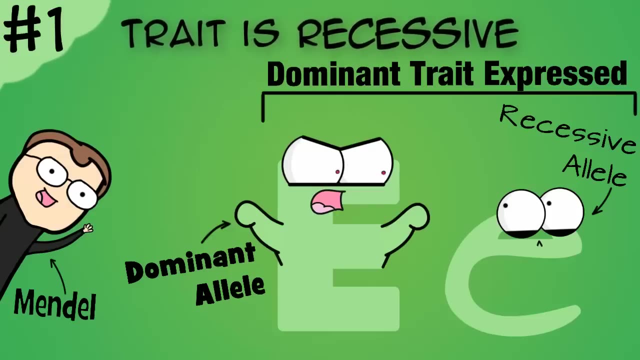 one about this trait being tracked is that it's recessive Recall that in typical Mendelian inheritance, dominant alleles, if present, will lead to the expression of dominant traits. Recessive alleles only are expressed when the dominant allele is not present. Now fact: 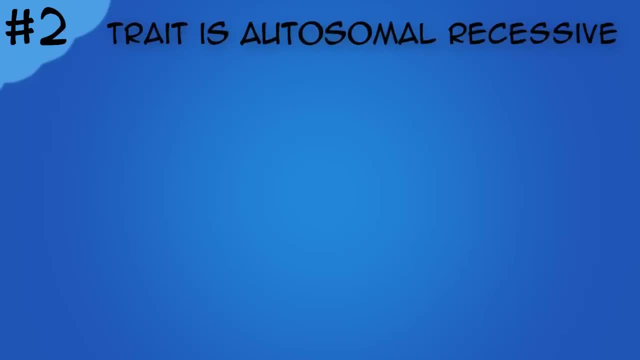 number two about this trait is that it is an autosomal recessive trait. Just a reminder that autosomal means a chromosome. that is not a recessive trait. It's a trait that doesn't have an autosomal recessive trait. Autosomal is an autosomal trait, It's not. 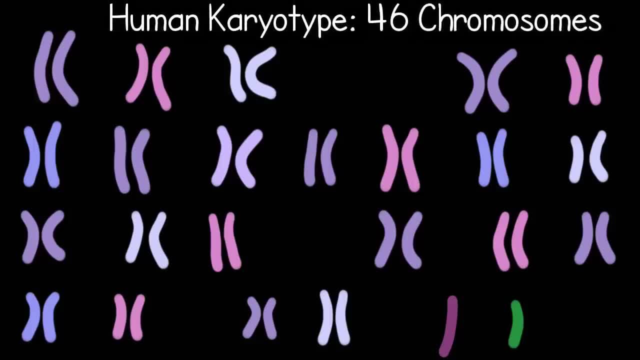 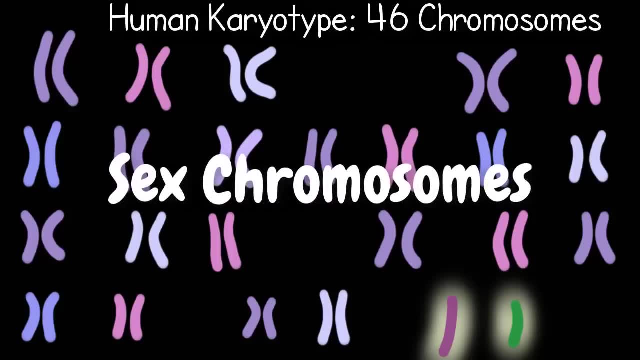 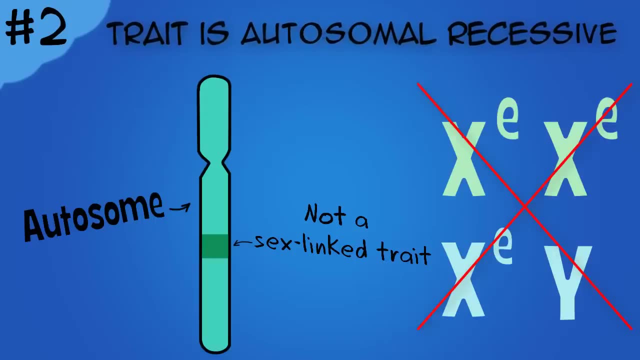 a sex chromosome. In human body cells there are 46 chromosomes. The first 44, 22 pairs are autosomes. The last two- one pair- are sex chromosomes. So this trait is not sex-linked since it is autosomal, and that means it does not need to be written as coefficients on. 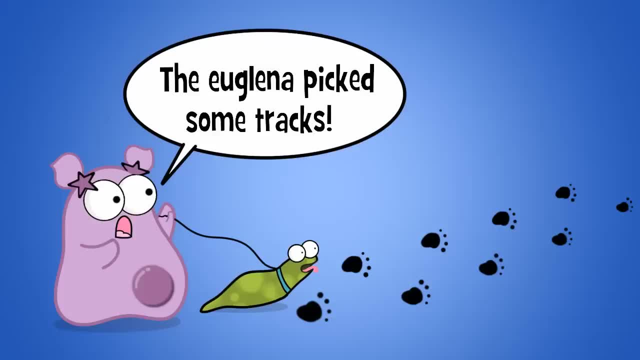 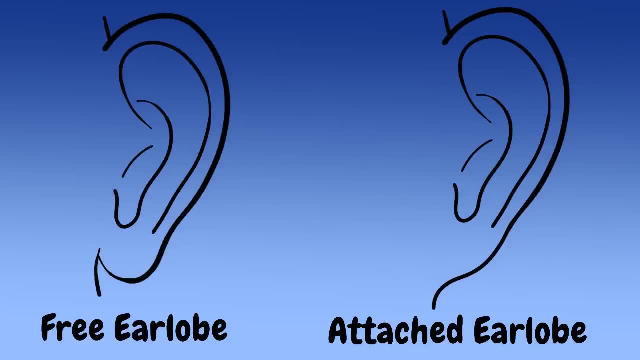 the sex chromosomes. So what is the trait we're tracking? Attached ear lobes. Yes, you might not realize it, but look around and you'll see that humans, they have free or attached ear lobes, Although we want to point out that there may be more than just these two categories for ear lobes. 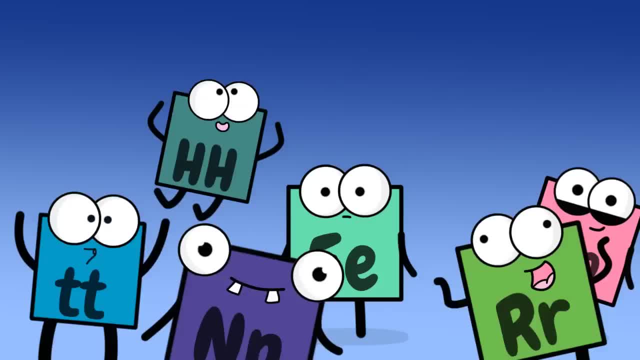 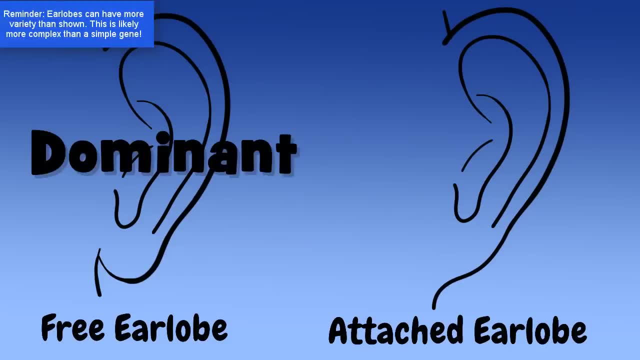 And while this example is used often in basic genetics, there's probably more to this than just one simple gene. For our example, let's assume a simple gene trait and that free ear lobes is dominant, meaning at least one dominant allele must be around. Attached ear lobes is recessive. 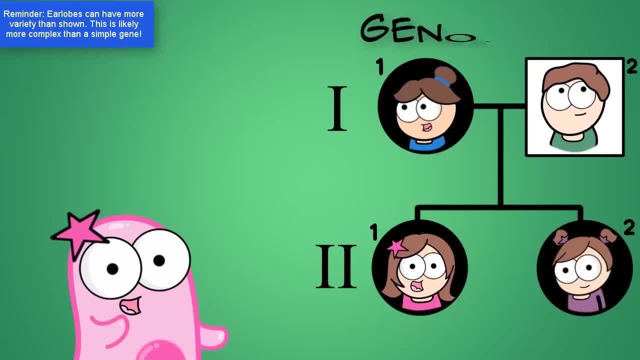 showing when no dominant allele is present. So if we were to put the genotypes next to each of these shapes, what would they be? Well, the shaded ones would be easy, because we just mentioned that attached ear lobes is recessive, showing when no dominant allele is present. 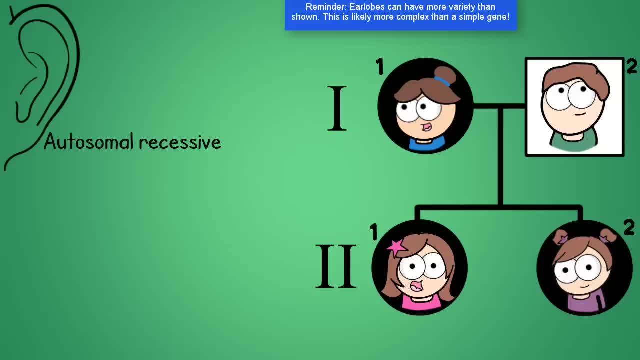 Attached ear lobes is the trait we're tracking and it's an autosomal recessive trait. So if we use the letter E, then these shaded shapes must be lowercase e, lowercase e, Any capital dominant letter and the individual would have to have free ear lobes and not 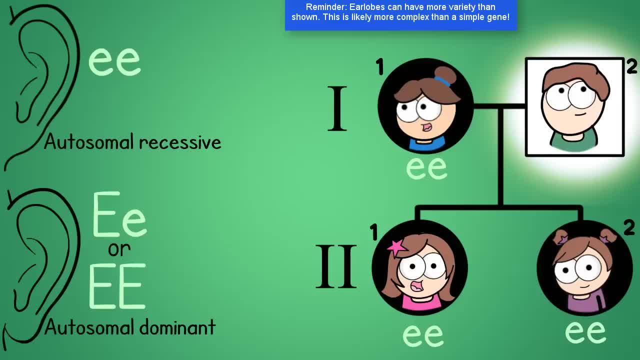 be shaded. So let's look at individual 2 in the first generation, That's our father. He's not shaded, so he can't be little e little e What about big E, big E? Well, there's a problem. 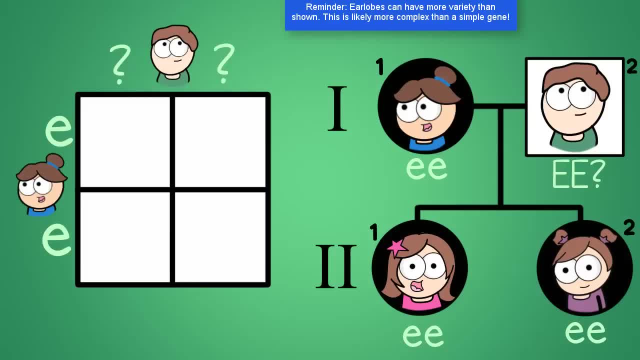 One child must get an allele from each parent. so if I received a little e from my mom, then I had to get the other little e from my dad. Therefore he can't be big E, big E or he'd have no little e to give. His genotype must be the heterozygote genotype: big E. 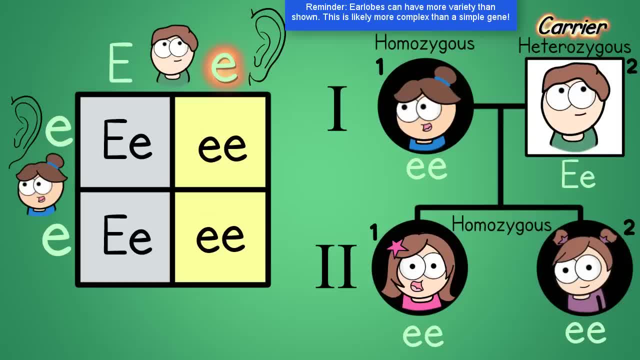 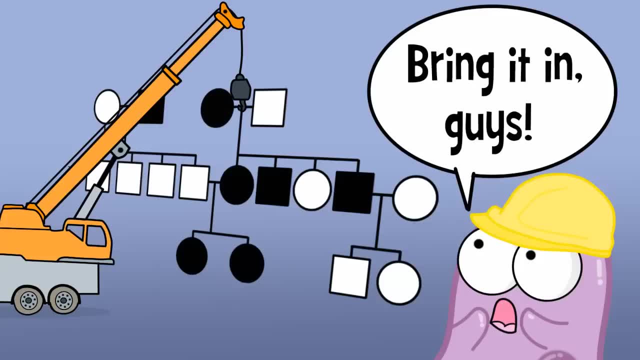 little e. He's what we call a carrier, though He still has a phenotype of free ear lobes because of that one capital, but he carries the lowercase allele. Now, that's just one tiny pedigree. Let's look at a big family reunion. Um, well, an imaginary one, because I have to confess. 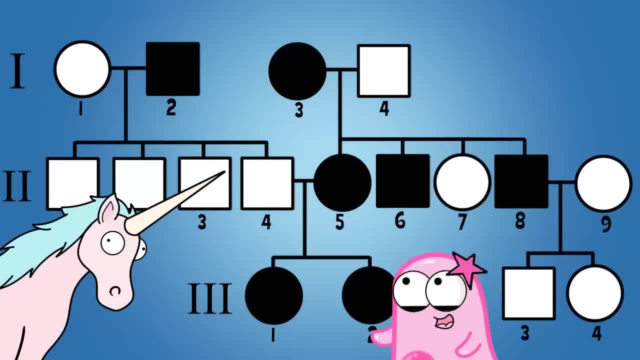 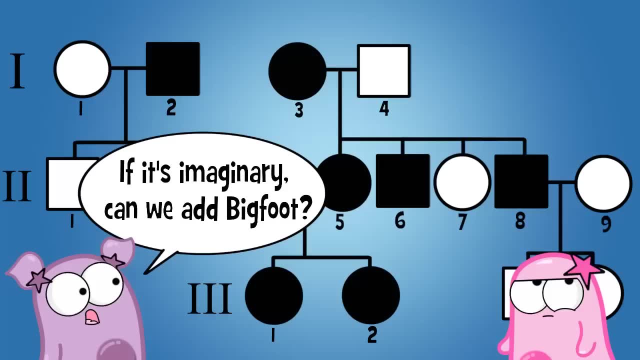 I don't really know whether our relatives have free or attached ear lobes. I thought about sending a survey to them, but it just felt a little awkward. So here we go, Big, giant imaginary family of relatives. Okay, just to make sure you understand this, how many siblings does my dad have? Well, 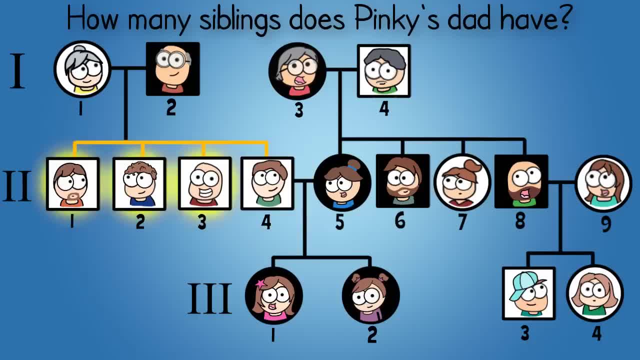 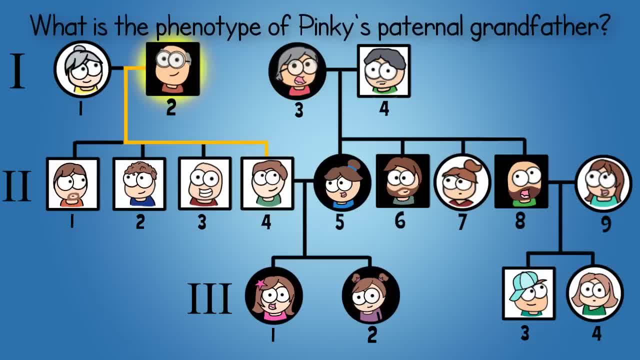 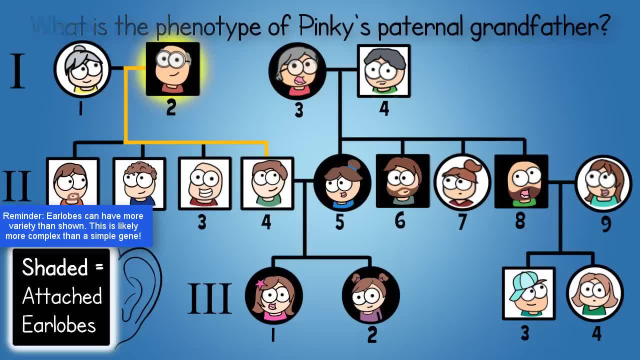 And what's the genotype of my paternal grandfather? Well, look, Here's my dad, Here's my dad's dad. That would be my paternal grandfather, Because his square is shaded. that means his phenotype is attached: ear lobes, Okay, so let's go ahead and label all these shaded shapes with the genotype little e little. 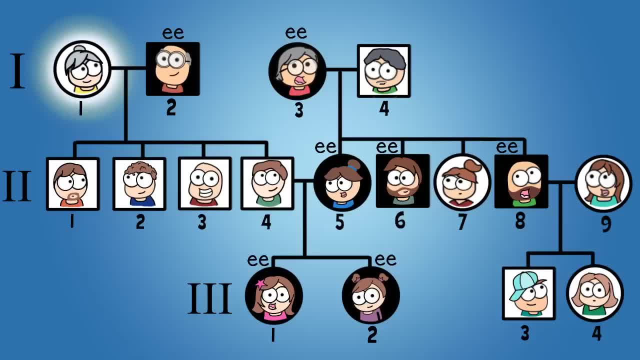 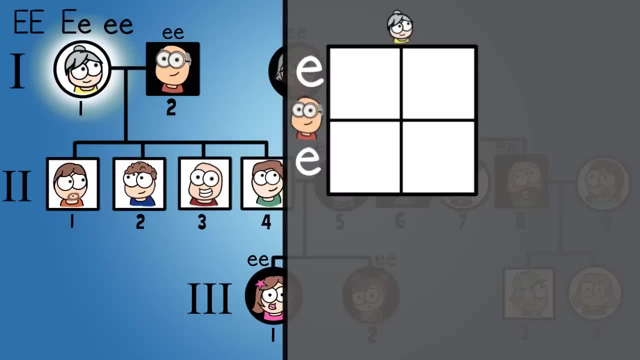 e, since we know that's the trait we're tracking. Now take a look at generation 1, individual 1.. That would be my paternal grandmother. What's her genotype? We know it's not little e little e I'm going to use the genotype of my mother. not little e little e. But 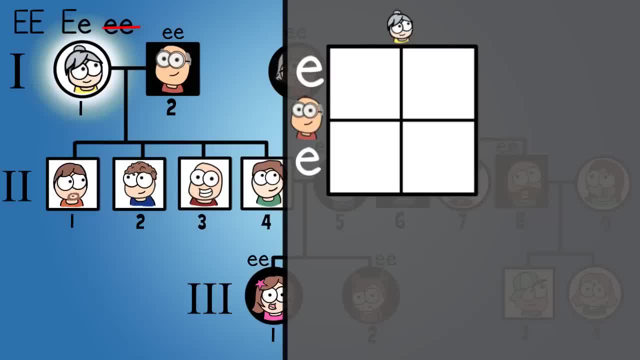 we know it's not little e, little e, little e. So now say, oh, you're my mother and I'm the physical E little e, or her shape would be shaded. But if we went with big E, big E could that. 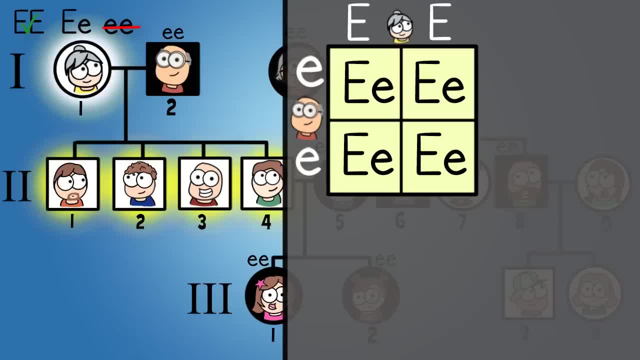 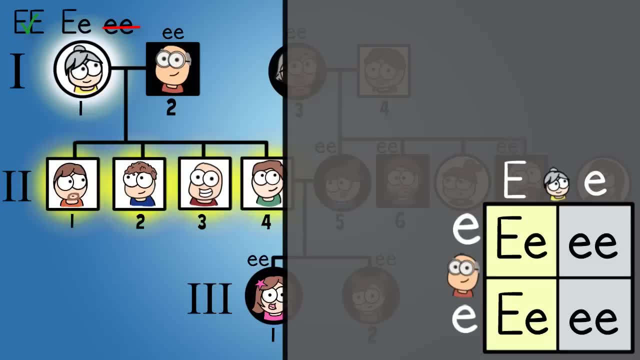 still work. Yes, all the offspring could get a big E from her and a little e from my grandfather. But what about big E little e? Would that work too? Yes, because the children could still get a big E from her and a little e from my grandfather. It may be less of a probability. 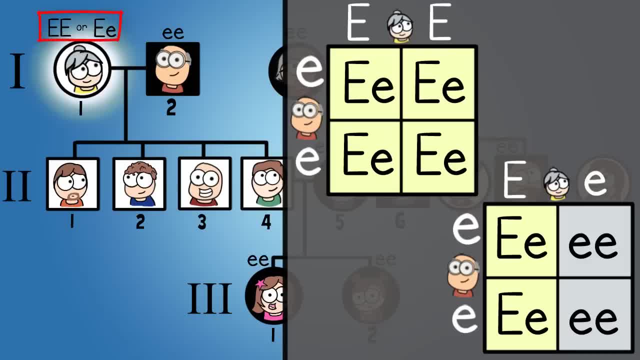 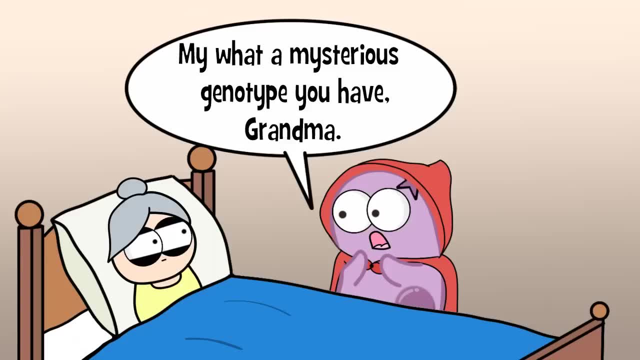 but it's possible, and therefore we must list both, that she is a big E, big E or big E, little e, because we don't know All the offspring of my paternal grandparents, though they're going to have to be big E, little e. Remember, they have to get an allele from 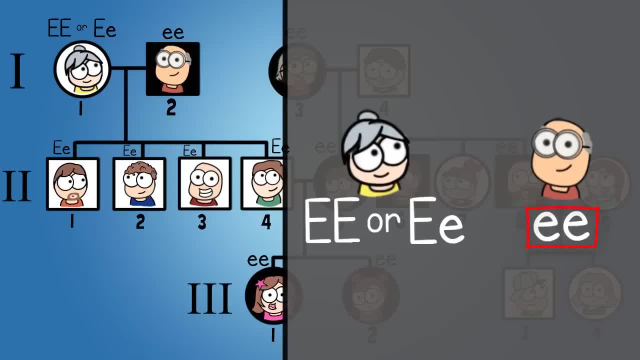 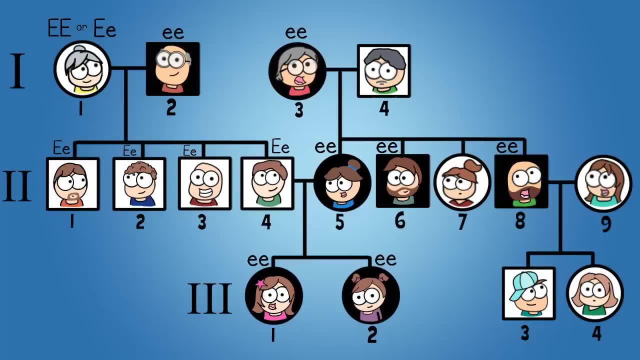 each parent, and that means they're going to have to pick up that little e from my grandfather. They will be heterozygotes and that's the only option here: Pause this video and try to solve the right side of this pedigree now. 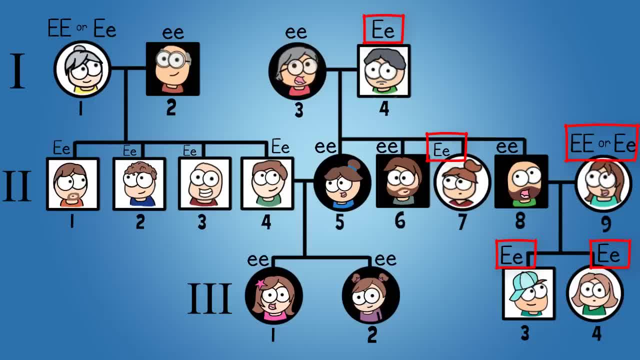 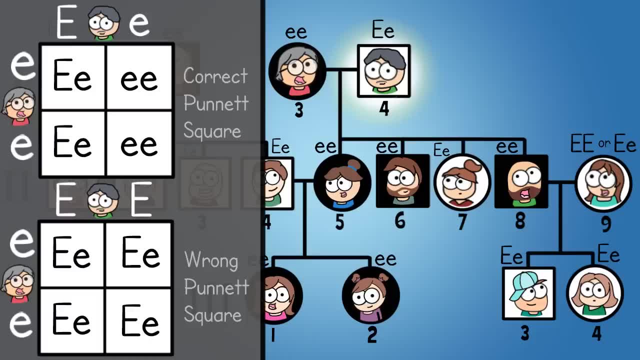 Ta-da Imaginary family done So how'd you do? Well, here are some of the tricky ones. Did you see that Generation 1, individual 4, has to be a big E? Would that be a carrier? only Because if not, then the shaded individual children would. 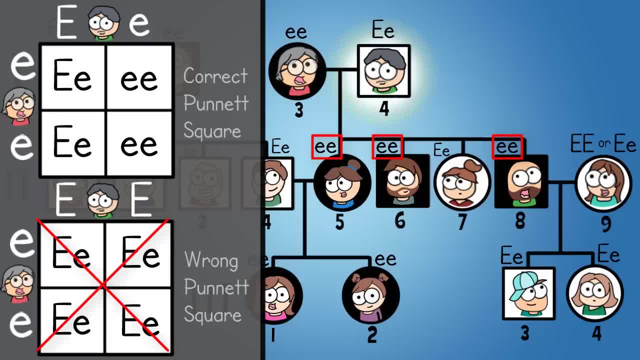 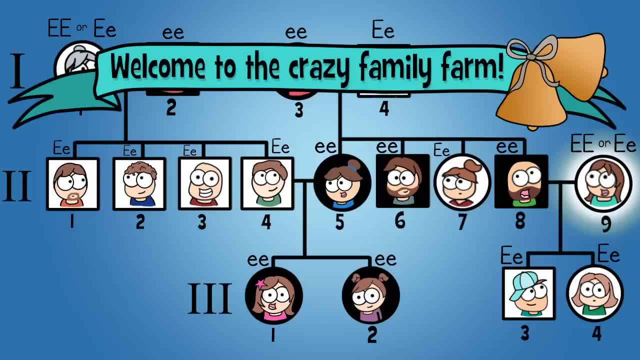 not be able to get the little e- little e that they have, because they have to get a little e from both parents. How about individual 9?? This female married in, but that's not the reason that she can be either big E- big E or big E- little e. If you look at the children, 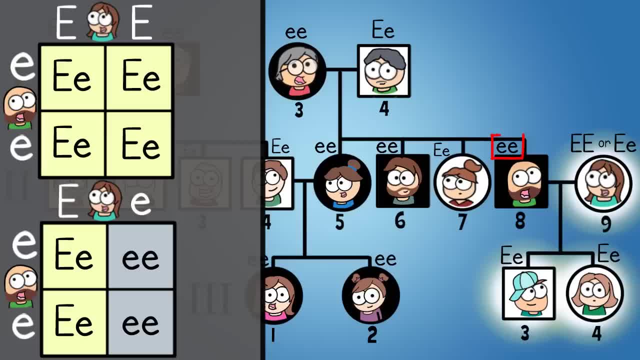 they aren't shaded. so while they will have to get a little e from number 8, as that's all number 8 can give, the other capital letter can be obtained from number 9, regardless of whether she's big E, big E or big E, little e. Remember one option may be more likely. 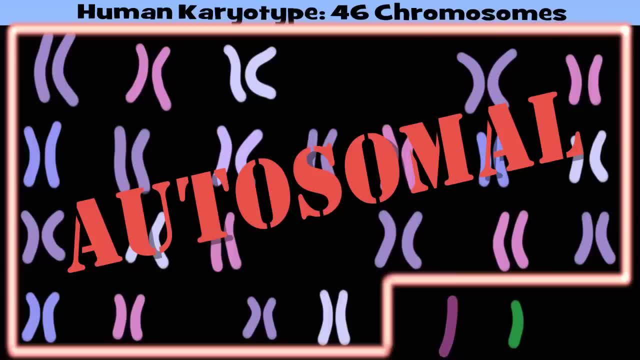 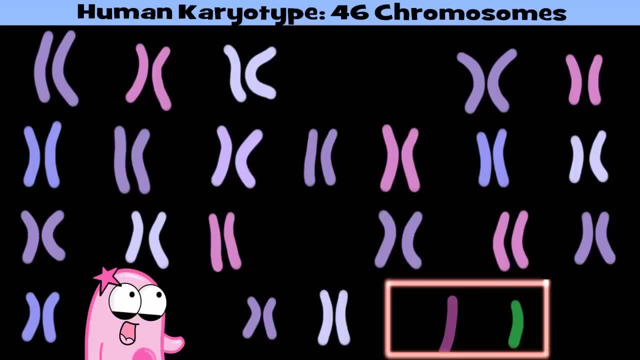 but if it's possible, you need to include both. Now remember how we made a big deal about how this was an autosomal pedigree. Well, what if you're dealing with a sex-linked trait and therefore a sex-linked pedigree? There are a lot of sex-linked recessive traits: Colorblindness and some male patterns of baldness. 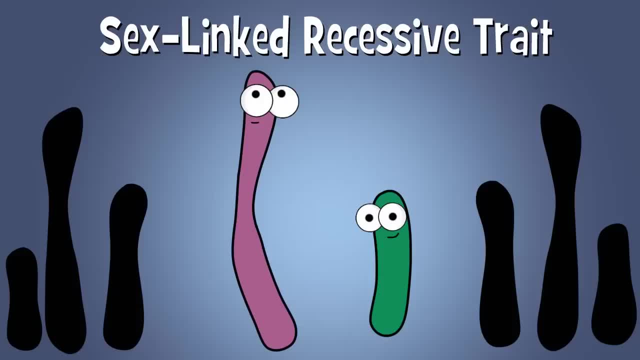 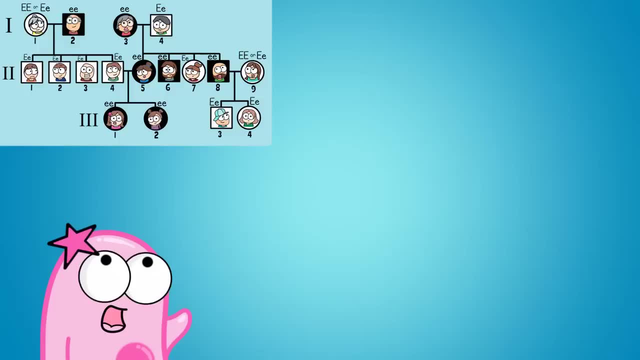 can be sex-linked. Let's pretend now that we're told this is a sex-linked recessive trait. I'm going to keep the old labeled pedigree here that showed an autosomal recessive trait, just for comparison. but now here's a brand new sex-linked pedigree. First of all all. 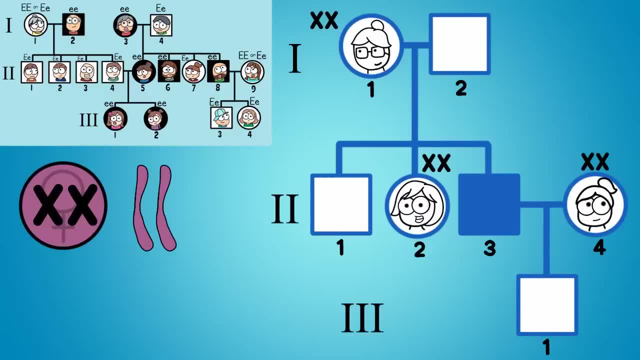 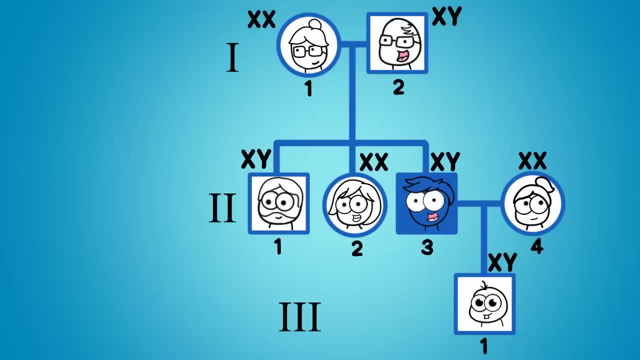 the females should have an XX to indicate two X sex chromosomes by them. Remember females have two X chromosomes. Males should have an XY to indicate an X and Y sex chromosome. That's always a good thing to do first. Now remember that we were told this pedigree is tracking sex-linked. 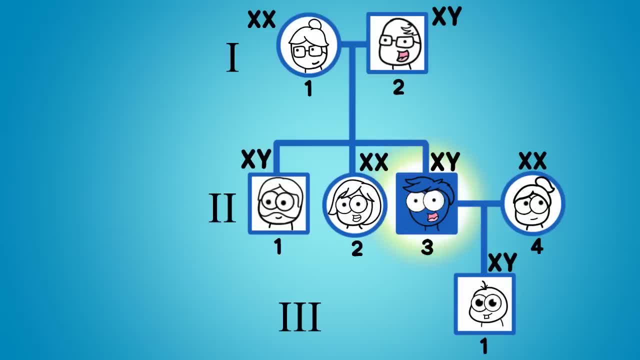 recessive traits. so the shaded one here has the sex-linked recessive trait. A reminder from our sex-linked video about how this works: Let's use the letter R for an allele. Recall that females that do not have the trait can be either this or this and the heterozygote. 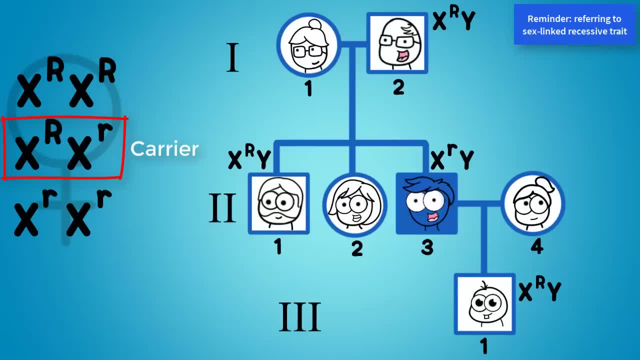 genotype. this is a carrier. She doesn't have the trait herself because of the dominant allele, but she's carrying it. Only a female, that is this- will have the sex-linked recessive trait. So if I'm looking at this pedigree, what would the genotype for individual 1 in? 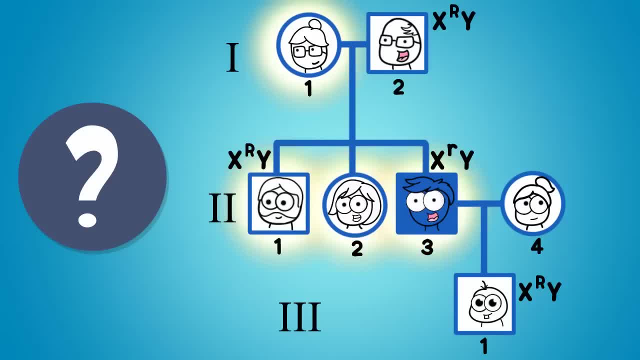 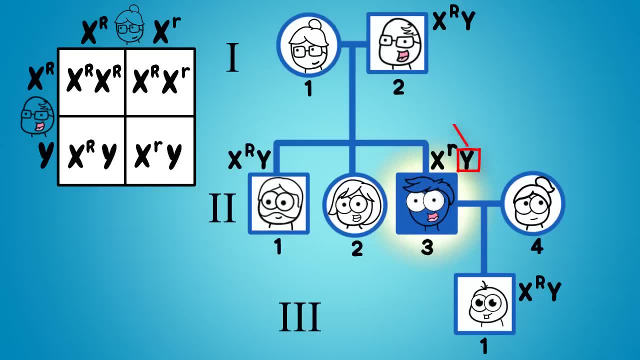 generation 1. be Well notice. here she has three children and one of her sons here is shaded. Where does her son get his Y sex chromosome from The father? Where does he get his X sex chromosome from His mother? Individual 1 doesn't have the trait or she would be shaded. 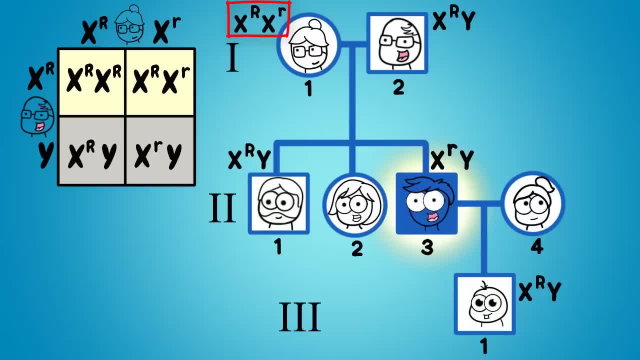 But she must be a carrier. if her son received an X chromosome with a recessive allele on it, What about individual 2 in generation 2?? Well, she can be this like her mother, But look, she could also be this, because it's possible to get one of those from each parent, If it's. 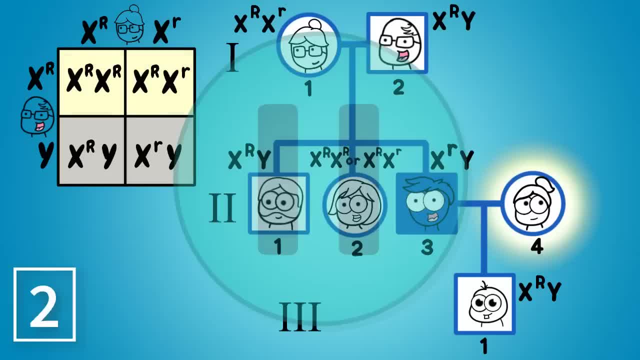 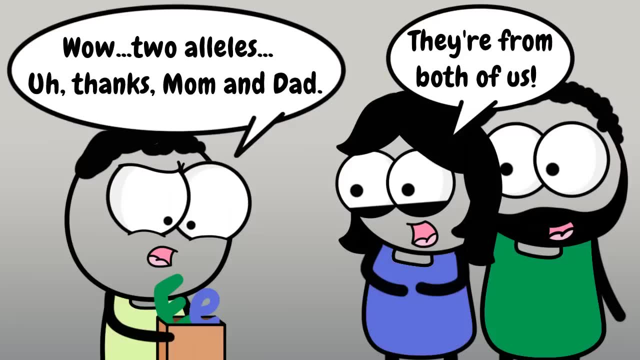 possible, you must include it Now. pause the video and try the last female. How'd you do Remember? the key here is to always check and make sure that when you look at a child, they have to be able to get one of their alleles from each parent. Now remember that both of 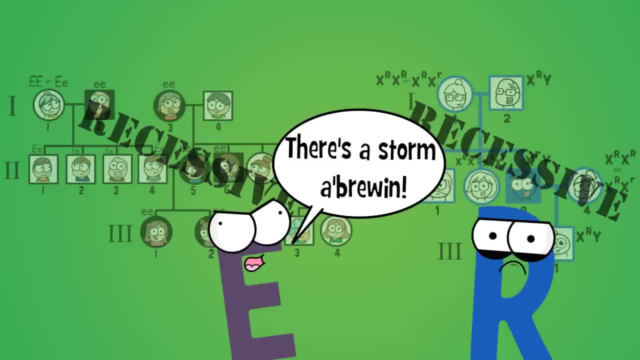 these examples were recessive. It doesn't have to be that way. On our handout you can try one that follows an R. So what about individual 2 in generation 2?? Well, she can be this like her mother, But look, she could also be this, because it's possible to get one of. 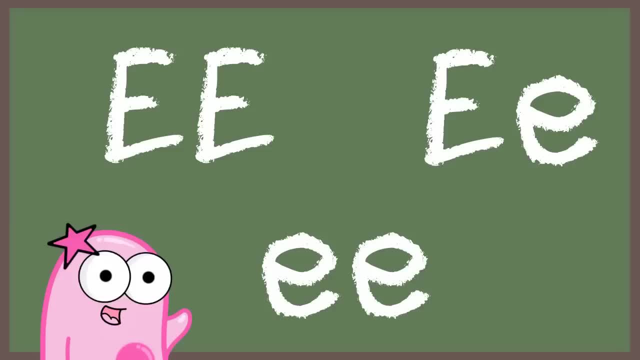 those from each parent. Remember the key here is to always check and make sure that she has an autosomal dominant trait. If it's a dominant allele that you're tracking, remember it would only take one dominant allele for a person to have that trait. 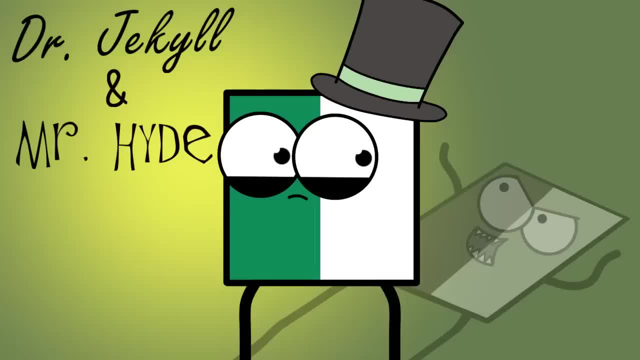 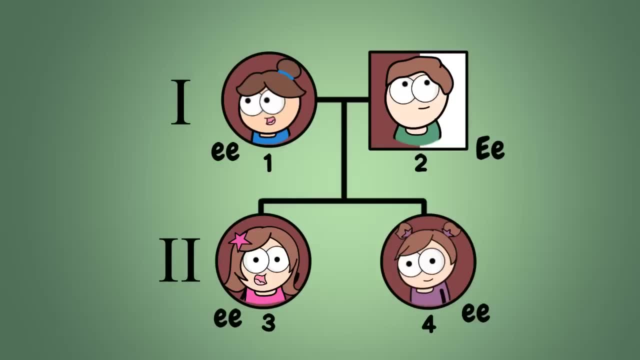 Another quick thing to point out is: sometimes you will see pedigrees that are half-shaded. Well, that's just awesome, because they're basically letting you know that the half-shaded ones are carriers. If I wanted to turn our first one into that… that half shading…. 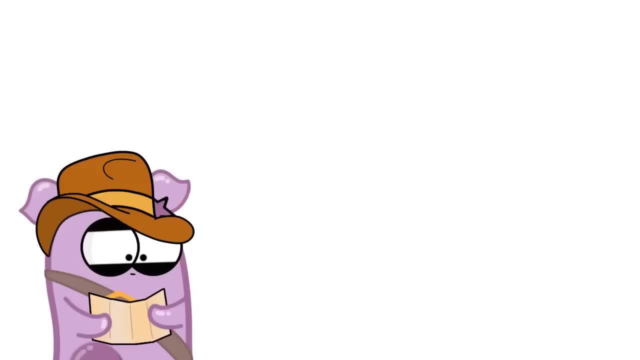 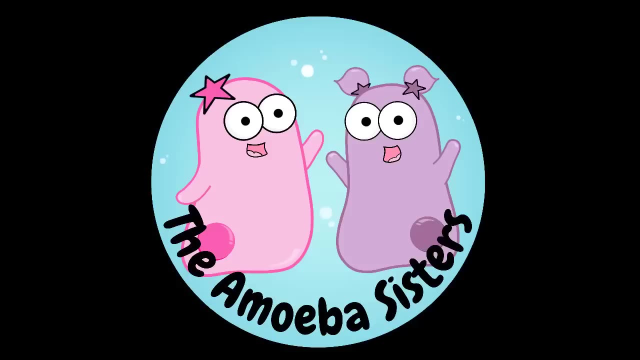 then it would look like this: Mapping and understanding pedigrees is important, especially as we continue to make advancements in understanding how genetic disorders affect us. orders are inherited. Well, that's it for the Amoeba Sisters, and we remind you to stay curious.